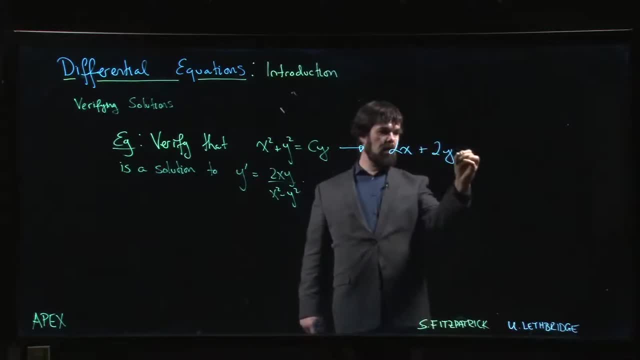 is 2y, but we're taking the derivative with respect to x, so we get a y prime. On the other side, the derivative of c times y is c times y prime. Okay, All right, Correct. So collect terms. 2x is equal to cy prime minus 2y y prime. Factor out that y prime. 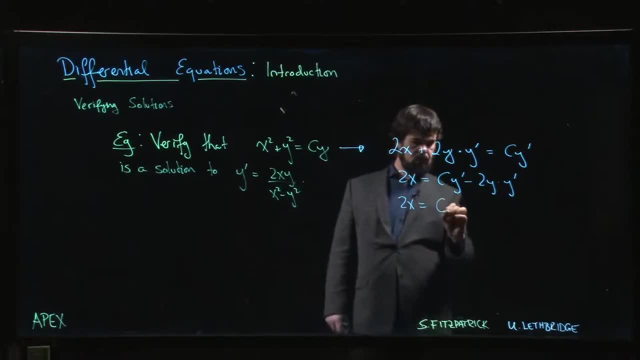 Okay, We get c minus 2y times y prime. Okay, C minus 2y times y prime. Okay, Well, c h. Well, x plus 2y… Or y plus 2y 2y. 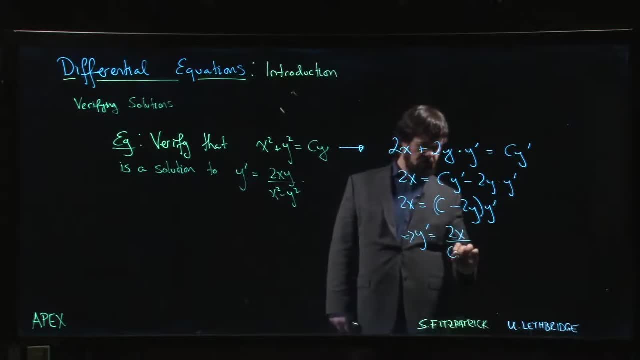 I'm sorry. 2x over c minus 2y. Okay, All right. Well, what do we do with that? Is that the same as this? I don't know, It doesn't look the same, does it? It looks rather different. 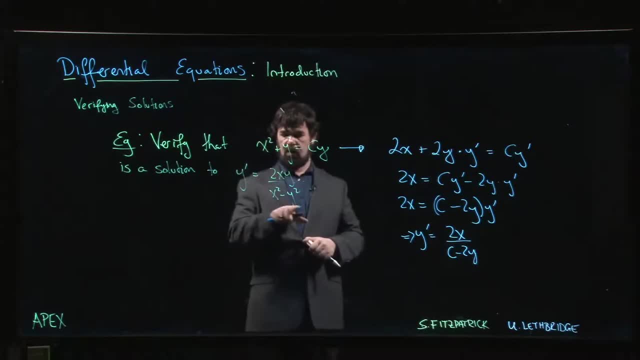 So now we have to think how do we solve that x squared minus y squared? Can we manipulate things? Can we get this to work? So let's see What can we do. We could try to eliminate that constant c. Maybe that's the way to go. Why not? Let's try it, Let's see what happens. 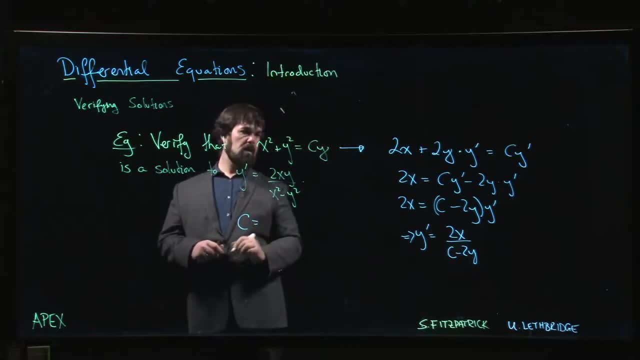 c is 1 over y times x squared plus y squared. Okay, So if I did c minus 2y, well, that would give me 1 over y times x squared plus y squared minus 2y, 1 over y. If we multiply top and bottom by y here, take the x squared plus. 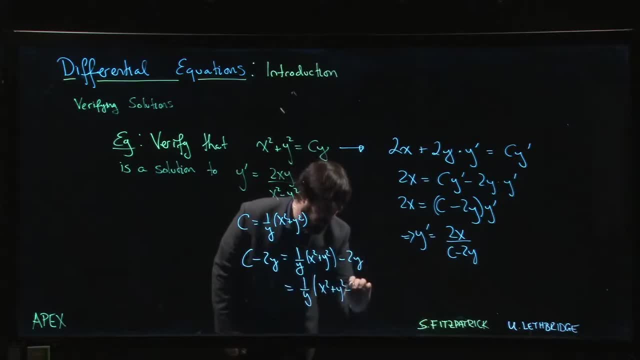 y squared minus. so 2y squared over y, right Minus 2y squared. Ah, interesting. This becomes x squared minus y squared over y. So this is 2x divided by 1 over y times x squared minus y squared. Multiply top and bottom by y. We.